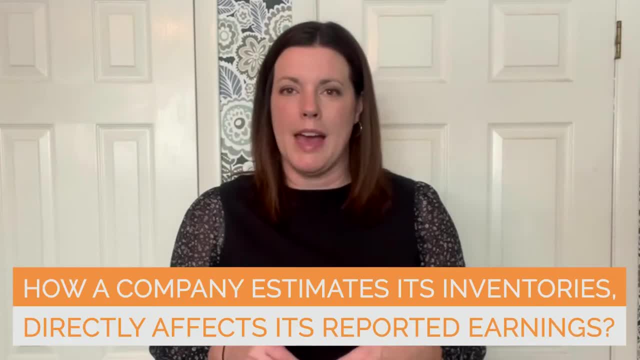 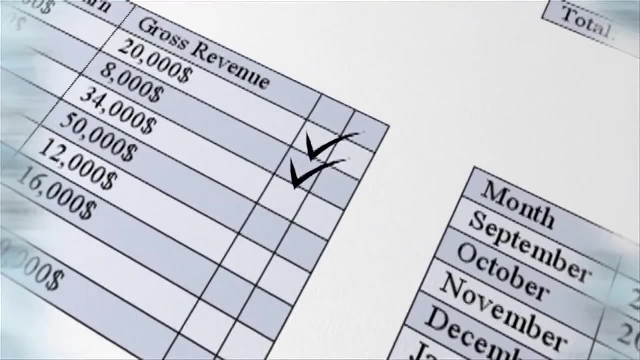 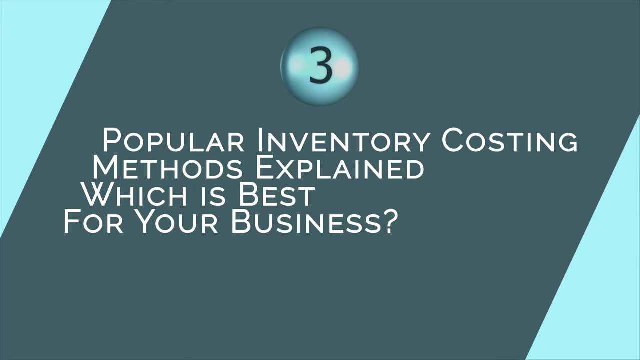 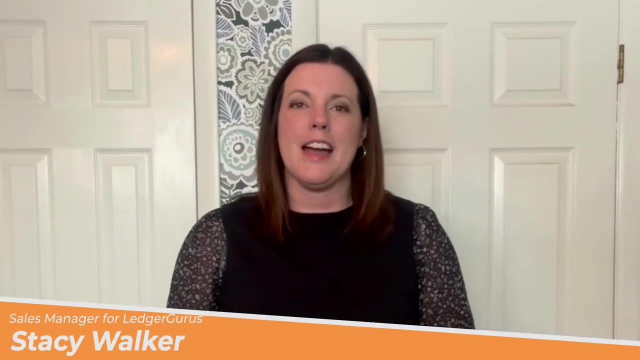 Did you know that the way a company values its inventory directly impacts its reported income and general financial health? That means that, without cooking the books at all, the method you use to calculate cost of goods sold can cost you more or less in taxes. Hi, I'm Stacy with Ledger Gurus and today I want to tell you about three of the most common. 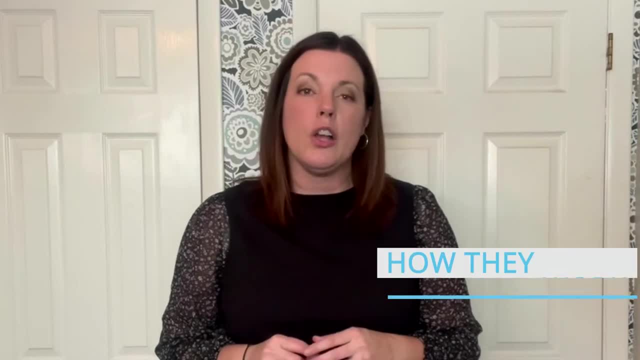 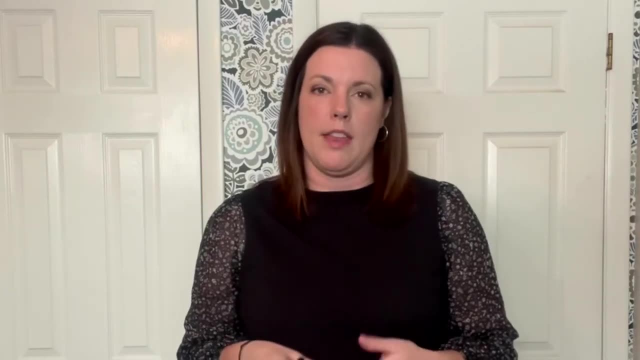 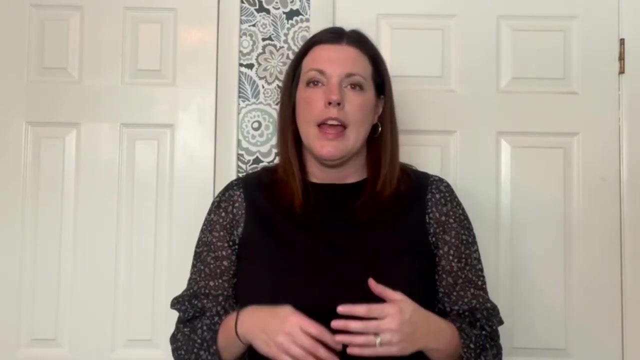 inventory, costing or valuation methods. I'll show you how they work, talk to you about their pros and cons and give you examples of which kinds of companies would benefit from each method. First, let's backtrack for just a quick second and discuss inventory systems. An inventory system is: 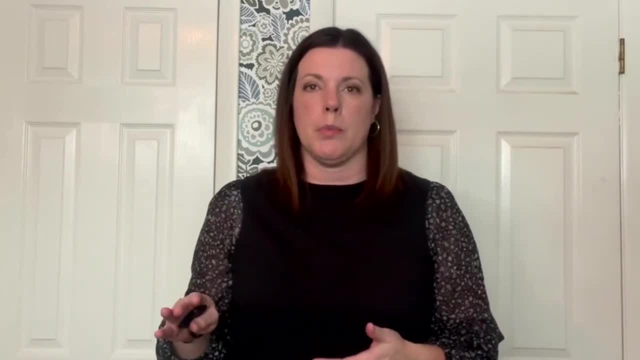 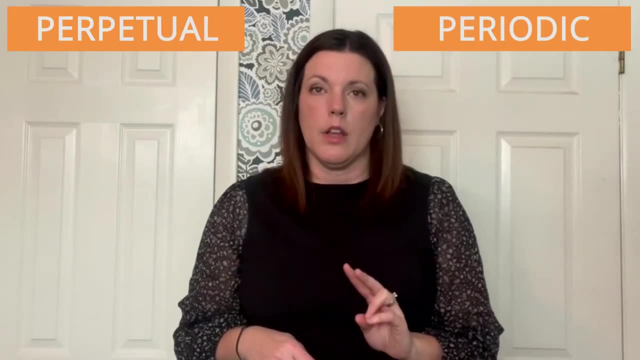 the system you use to track your inventory as it moves through the supply chain. There are two systems. The first is perpetual inventory system. The second is periodic inventory system With a. With the Perpetual Inventory System, inventory and cost of goods sold accounts are updated. 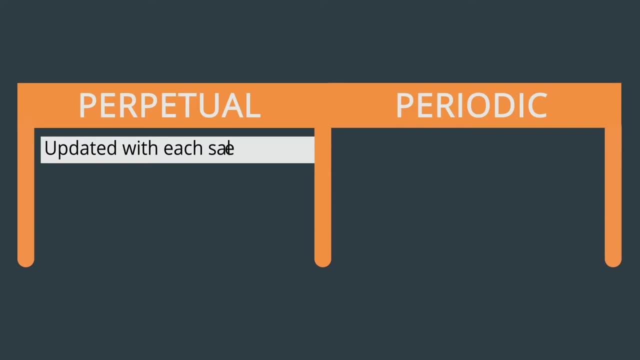 with each sale, or perpetually. With the Periodic Inventory System, inventory and cost of goods sold accounts are updated periodically. Small businesses using straightforward accounting procedures typically choose to use the Periodic Inventory method because it's super simple, It doesn't require a high level of operational maturity and it can still provide accurate 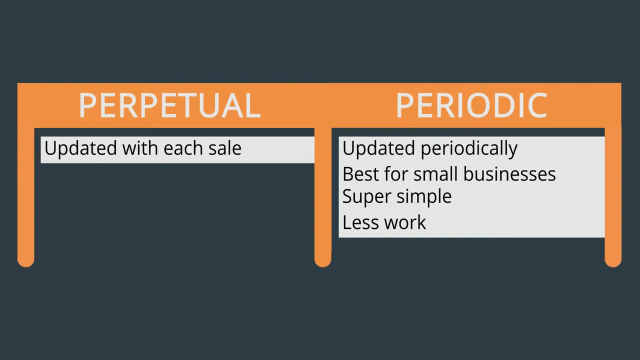 financials with less work On the flip side. keep in mind that this method is also less timely. As your business grows, you may choose to switch to the Perpetual method for a couple of different reasons. First, the balance in your inventory account is current at any point in time. 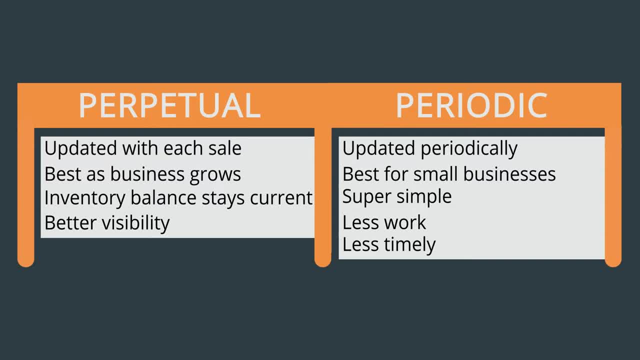 And second, it provides better visibility for a large volume of inventory transactions. Those companies using a Perpetual Inventory System will assign a value to their inventory with each sale. Those using a Periodic Inventory System will do so periodically, maybe once a month or 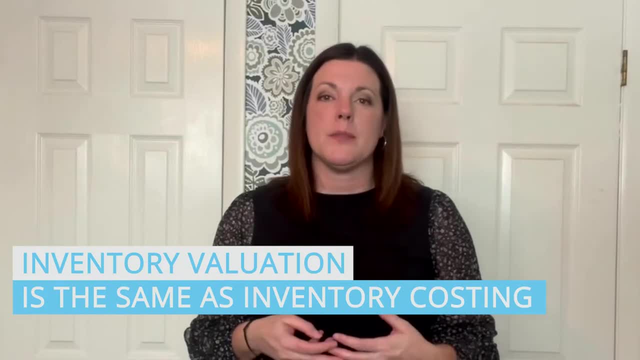 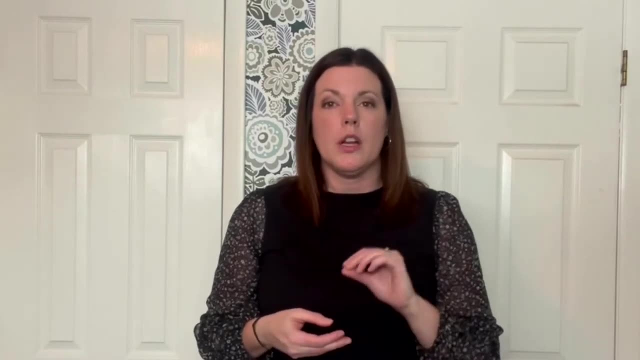 even once a year. Throughout this video, I will refer to this process both as inventory valuation and inventory costing. It's the same thing, just different words. In essence, you are putting a dollar amount on your inventory. This is how you determine the value of your inventory and the associated cost of goods. sold. Let's dive into three inventory costing methods, how they impact your business and the pros and cons of each. First up is average cost. Average cost is one of the most popular costing methods. It's simple: You divide the total cost of purchased items by the number of items in stock. 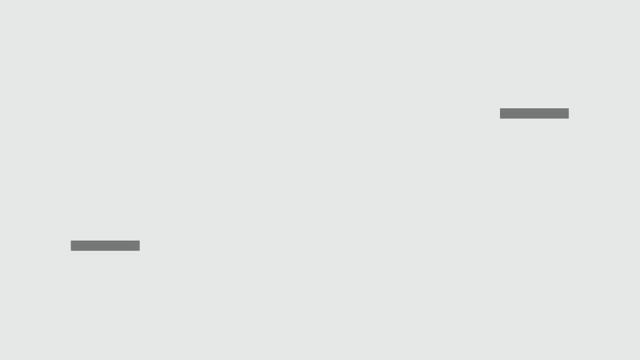 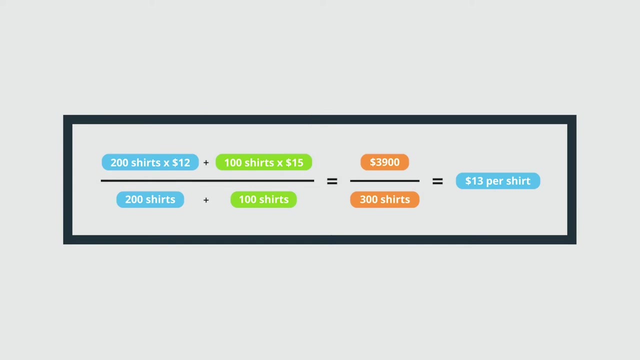 Let's look at an example. Say you own a custom shirt printing business. You make two purchases of blank shirts. The first purchase of 200 shirts costs $12 per shirt. The second purchase is for 100 shirts. that cost $15 a shirt. 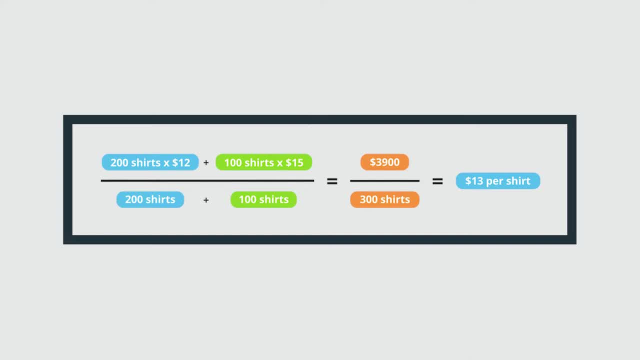 You now have a total of 300 shirts that you invested a total of $3,900 in. At the end of the week, you have sold 75 shirts, So how do you value your leftover inventory? Let's take a look. You assign the average cost of $13 per shirt to each of these buckets. 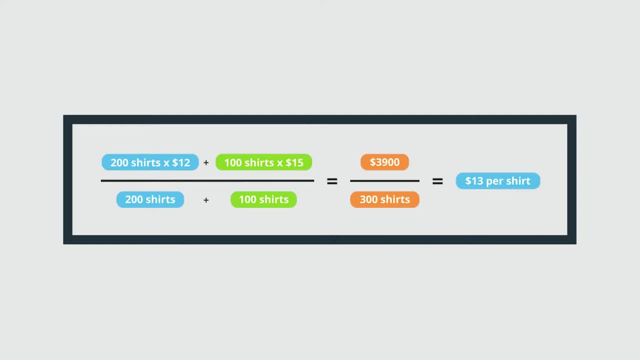 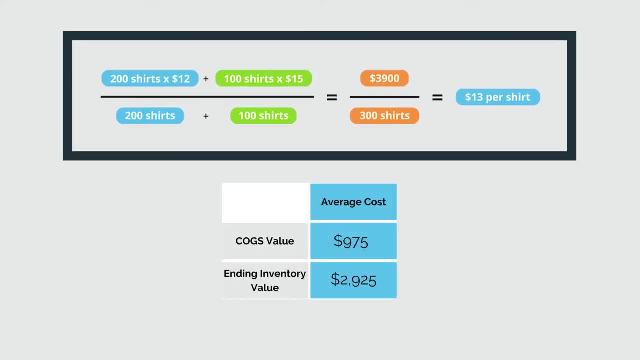 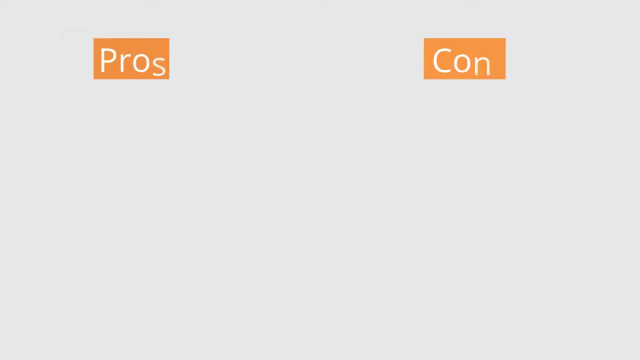 75 shirts sold and 225 left over in inventory. The average cost is $13 and after selling 75 shirts, the account balances will show $975 in cost of goods sold and $2,925 in remaining inventory. Pros to the average costing method include ease and simplicity to apply. the chances 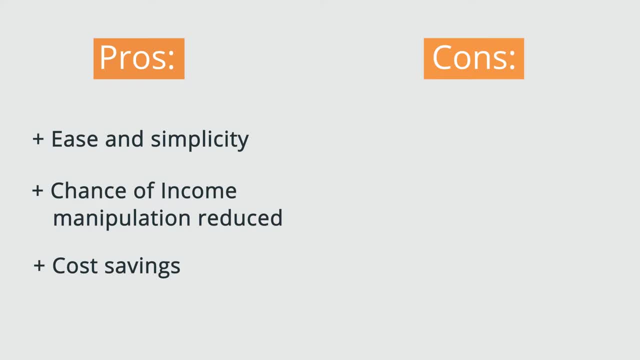 to buy and the cost savings associated with this method, simply because it requires a very small amount of time to maintain. On the other hand, some of the cons to this method would be: the inventory prices vary and pricing may not cover the cost of the more expensive units. 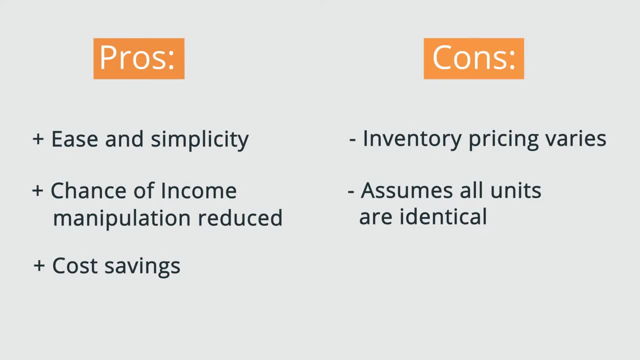 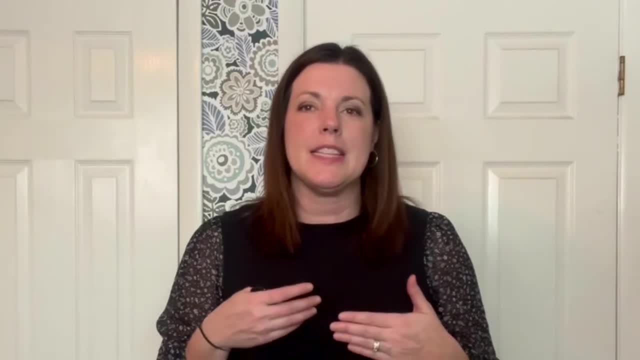 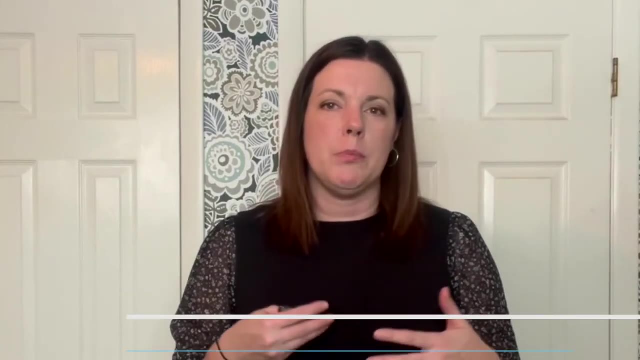 Also, there is an assumption that all units are identical, which is often not the case, causing mispricing. One major consideration of this costing method is that it can become significantly skewed over time. If you choose to use the average costing method, it would be really smart to do adjustments. 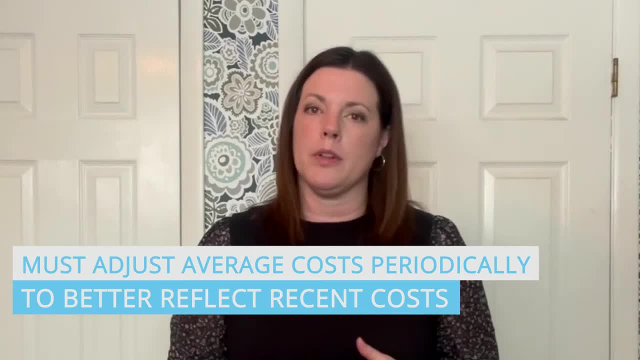 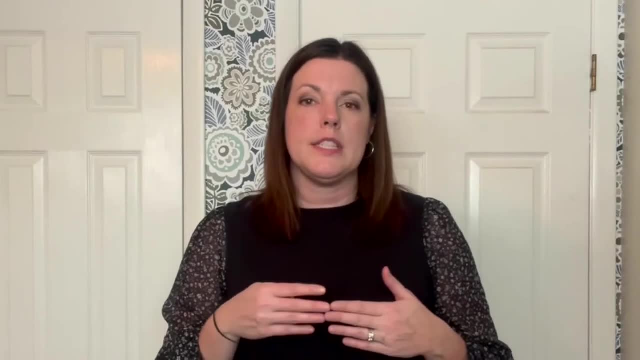 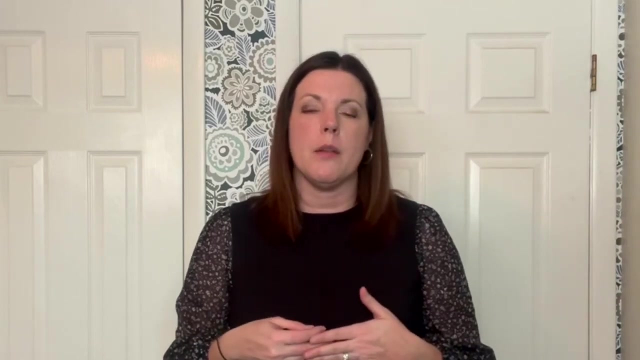 to your average costs periodically, at least every couple of years or so, to bring them closer to an average cost that more accurately reflects your recent costs. If your business deals with large volumes of very similar items or you do a lot of your own manufacturing, the average costing method might be right for you. 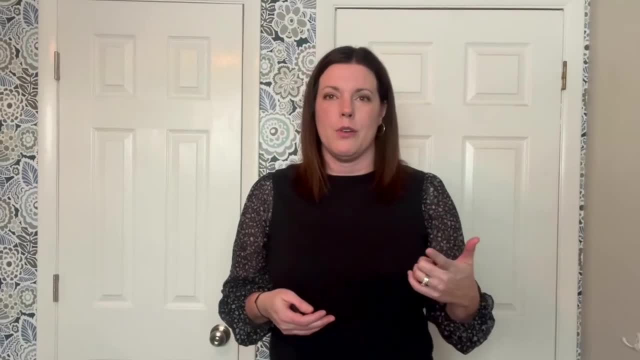 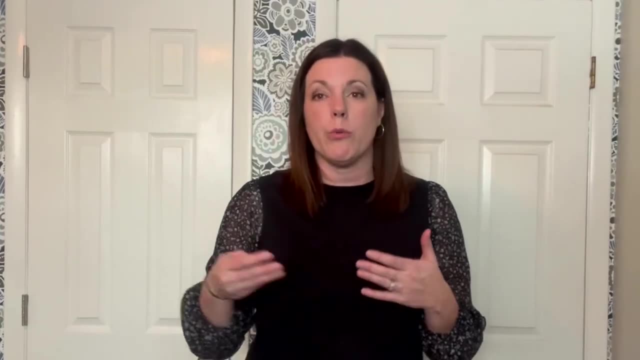 This brings me to our next two costing methods: FIFO and LIFO. When we are using FIFO or LIFO, we have to consider that small products bought in bulk are almost never assigned the cost they were originally purchased at. The exception to this would be large items like cars, appliances or expensive pieces. 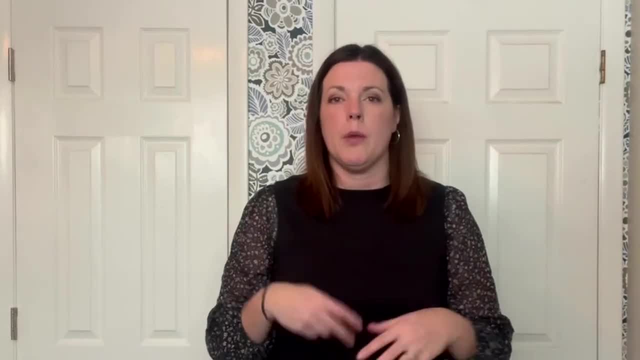 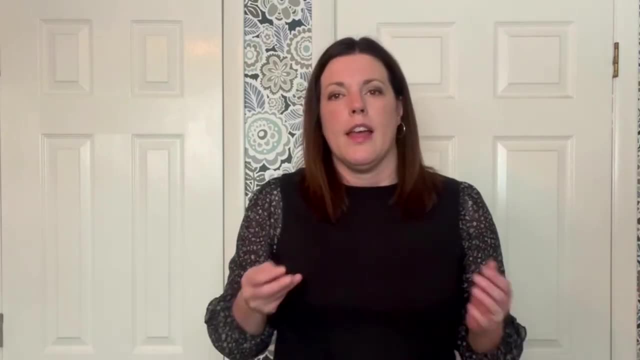 of jewelry, But in general they're all dumped into one bin and pulled out when sold. How do we know whether this particular item was bought at $12 or $15? Well, the fact is we don't. That's where FIFO or LIFO come in. 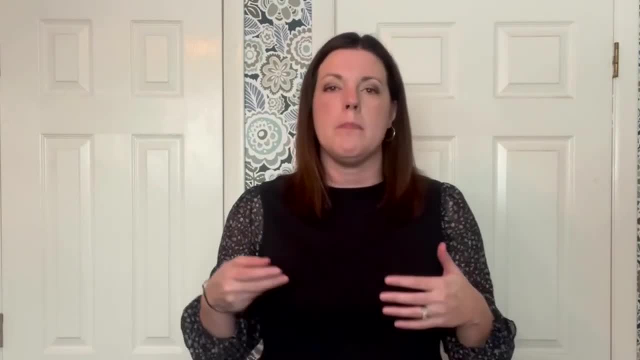 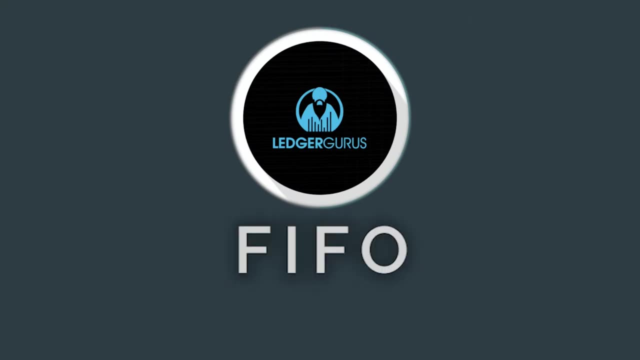 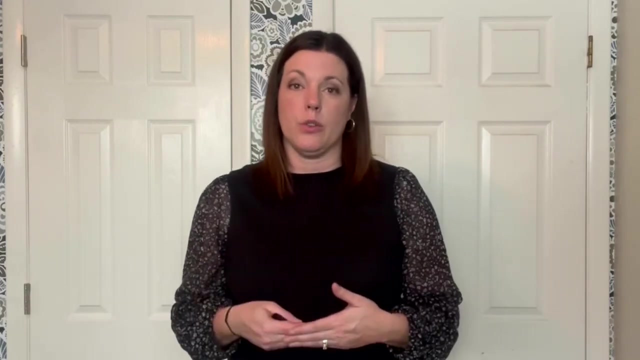 We place products in pricing tiers when they're bought and then make a general assumption on the order that those pricing tiers will be pulled off the shelf and sold. So let's talk a little bit about FIFO. Businesses that use FIFO record the oldest inventory items to be sold first. Thus, first in, first out, When inventory is sold, the oldest cost of an item in inventory will be recovered and then reported on the income statement as part of the cost of goods sold. We track how many items were bought at the oldest price tier and then use them all up. 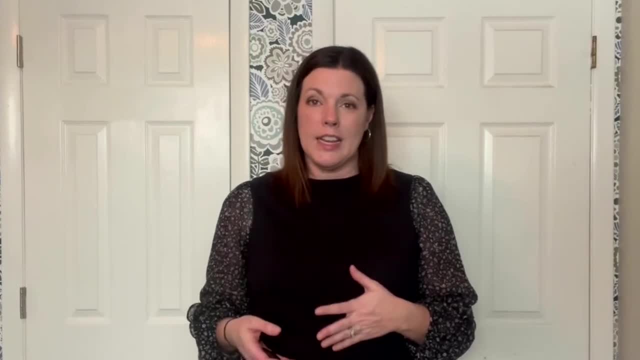 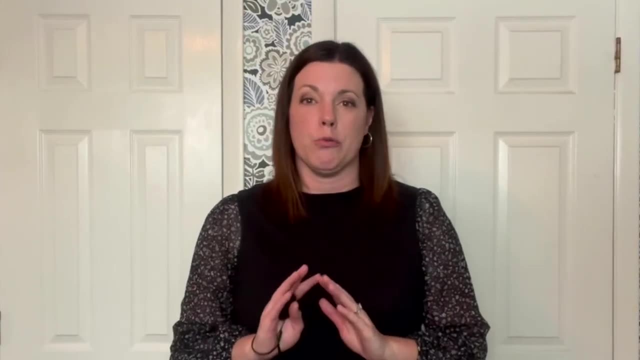 before moving on to the next price tier. For the sake of sanity, I really hope you're using an inventory management software if you're trying to use FIFO or LIFO, because this can get seriously crazy. Let's go back to our shirt example. 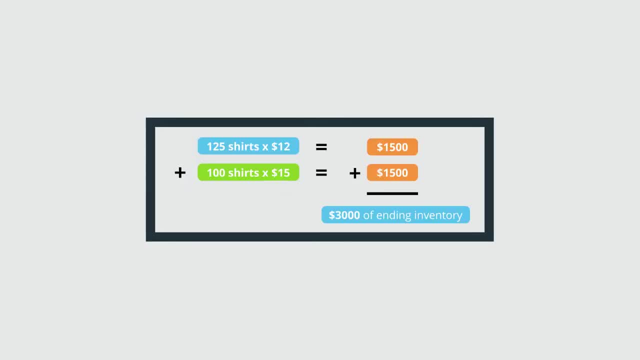 What is the FIFO cost of our shirts? Well, it's $12, because the first 75 shirts we bought cost $12.. So they are the first ones considered. Remember: first in, first out. This means that the cost of goods sold for 75 shirts at $12 a shirt would be $900.. 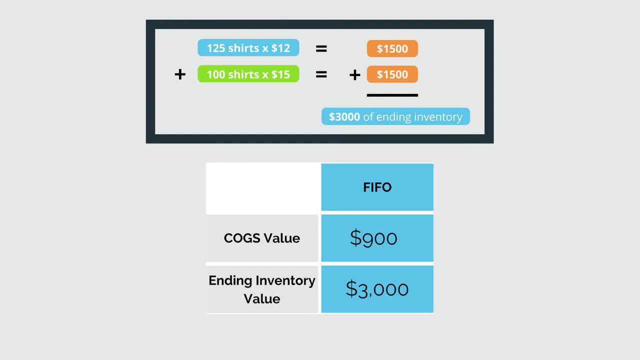 Those 75 shirts were taken from the oldest pricing tier- This can also be called a tranche, by the way of shirts. but there's still 125 left at that $12 price point, because we bought a total of 200 in that first tranche. 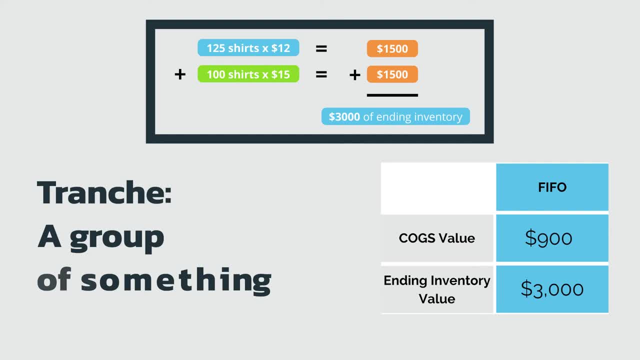 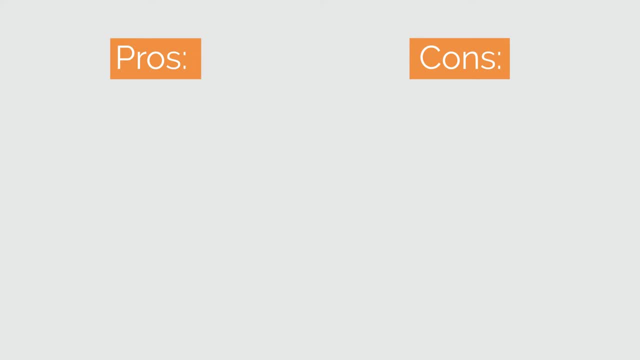 We also still have all 100 shirts of the second tranche at $15 per shirt. So our inventory balance is $3,000.. Pros to this approach would be that, since you are using often lower and older costs assigned to cost of goods sold, 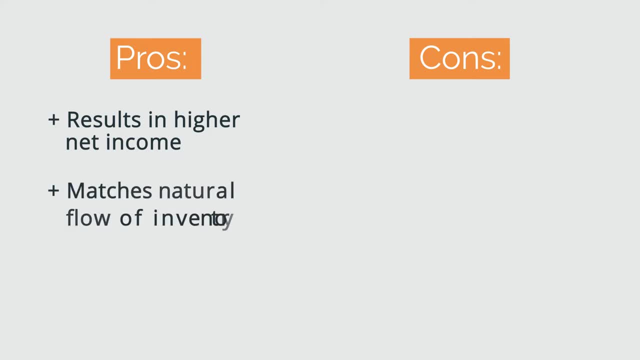 It results in higher inventory costs. It results in higher net income. It also matches the natural flow of inventory and is widely used and understood. Cons you might want to consider would be: you may end up in a higher tax bracket. Prices generally increase, which means the earliest purchase inventory had the lowest. 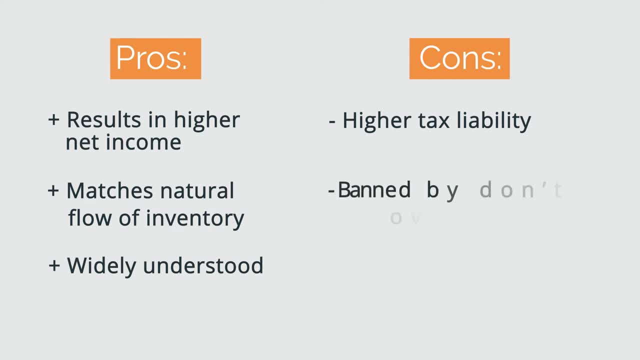 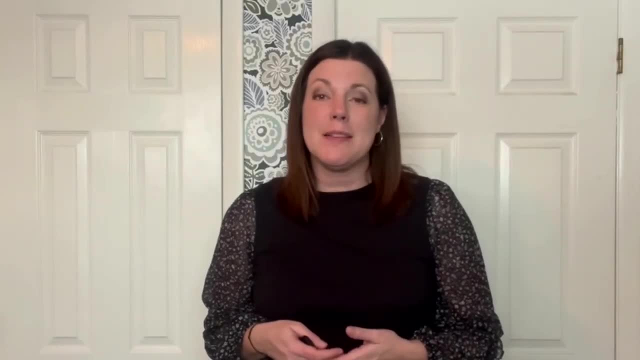 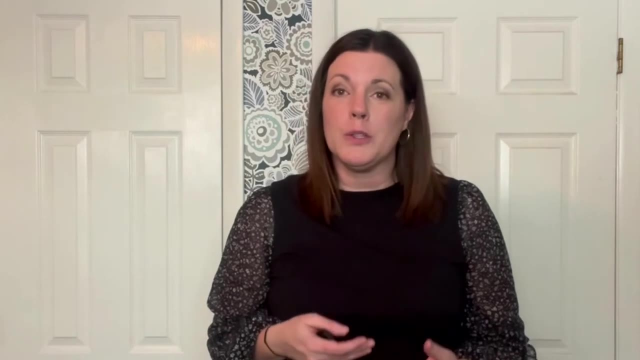 cost and will have a higher margin when you sell it. Also, since revenue and cost don't match, this can overstate your profits. FIFO is normally considered the costing method crowd favorite because it creates the most accurate picture. Think about it: Most businesses do want to get rid of their oldest items first and usually consider this. approach to be the costing method with the fewest issues to correct. in the long run, However, it does create the lowest cost of goods sold number when prices are rising, which can result in higher taxable income. Stay to the end of this video to find out more information about that. If your business deals with perishable stock or short demand cycles, FIFO costing method might be right for you. Lastly, let's chat about LIFO. LIFO is the opposite of FIFO and reports the most current prices as being the cost of goods sold. thus, last in first out. This means that when inventory is sold, the newest cost of the item in inventory will be recovered and reported on the income statement as part of the cost of goods sold, and the oldest prices will be what's remaining in ending inventory. So let's go back to our shirt example. 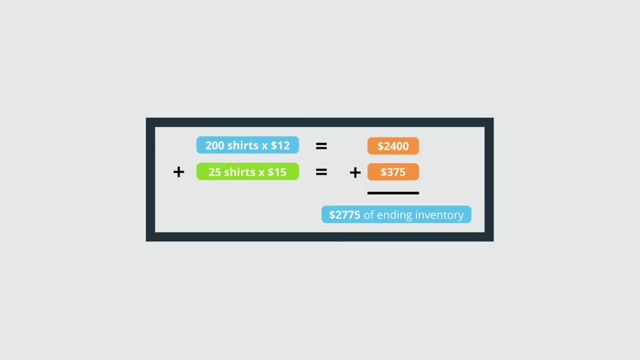 What is the LIFO cost of our shirts? Well, $15.00.. We bought all of our shirts because they were the last items we bought, so they're the first items that we'll sell. What does that mean for cost of goods sold in inventory? 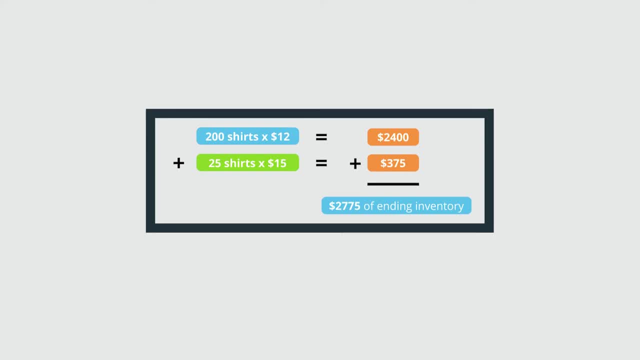 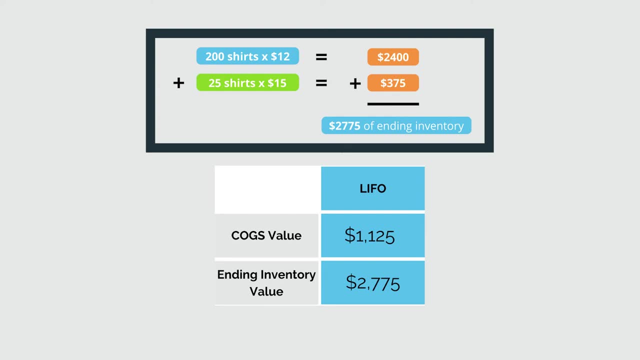 The cost of goods sold. for 75 shirts at $15.00 a shirt means that our cost of goods sold number would be $1,125.00.. Those 75 shirts were taken from our newest tranche of shirts, but there's still 25 left. 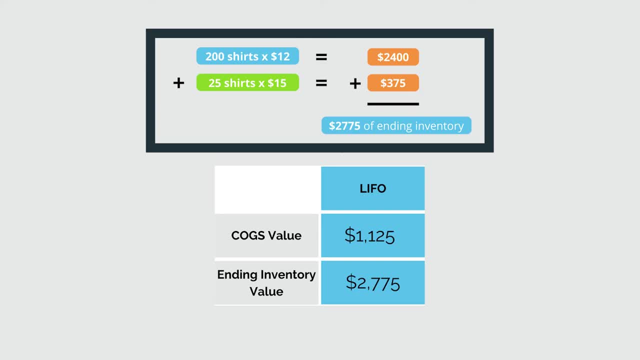 at the $15.00 price point because we bought 100 in that tranche. We also still have all 200 shirts of the older tranche at $12.00 a shirt. So our ending inventory is $1,125.00.. 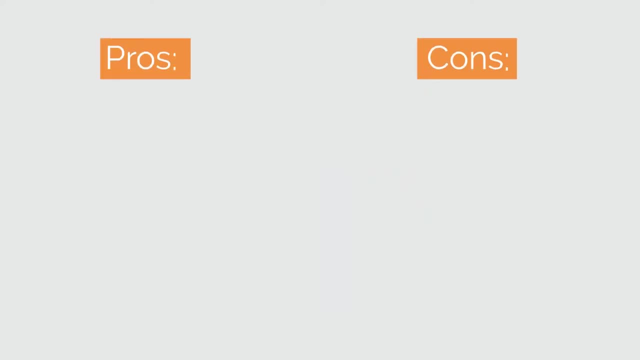 The cost of goods sold in inventory is $27.75.. Pros to using this inventory costing method would be that, during times of inflation, the cost of goods sold is higher, reducing the profit margin, which results in a smaller tax liability. It's also the most appropriate method for matching cost and revenue and is widely used. 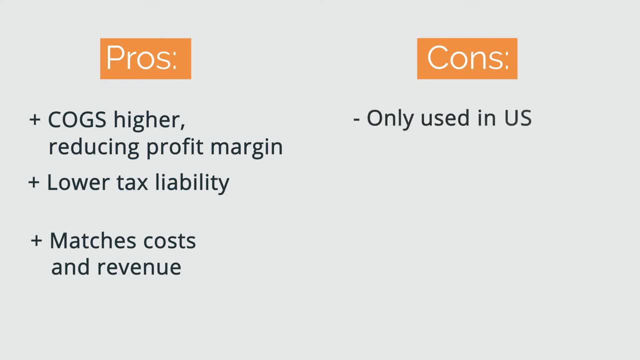 and understood Cons to consider would be that LIFO is really only used in the United States. It's governed by GAAP and is actually banned or restricted by certain organizations, Also because of the cost of goods sold in the United States. the cost of goods sold. 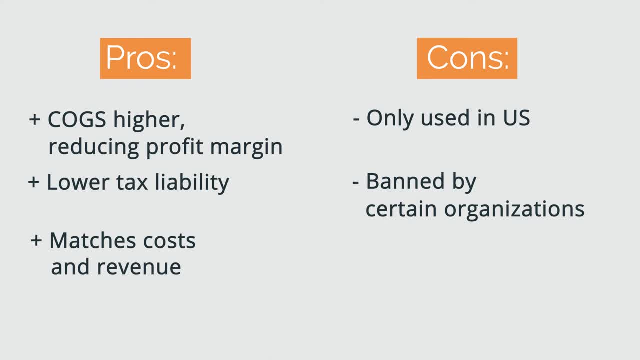 is higher Because inventory sold under the LIFO method has the highest cost of goods sold. the profit margin and income for the business is lower. This method can leave you with a majorly understated ending inventory balance, Basically, unless you're turning over 100% of your inventory before ever buying more. the first items bought never actually show as sold. So over time, as prices rise, these ending inventory balances become less and less representative of the actual value of the inventory Companies with relatively large inventories, such as the automotive industry or big retailers. 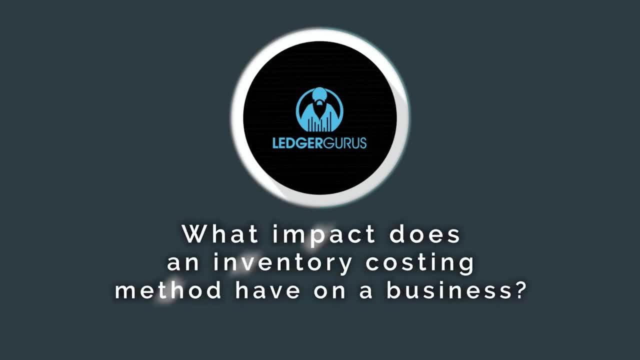 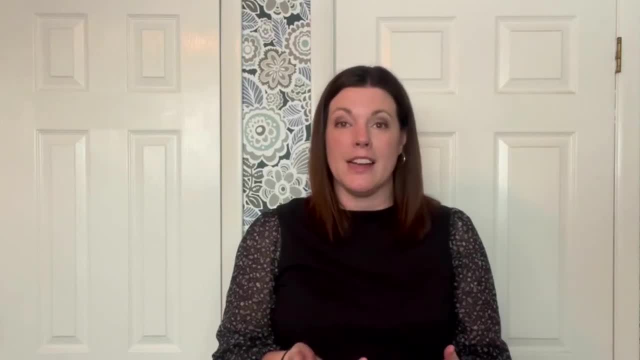 might consider using the LIFO costing method. Now that you know all about the different costing methods, you might be wondering what impact an inventory method has on your business. So let's return to this idea of how an inventory method can impact your business. 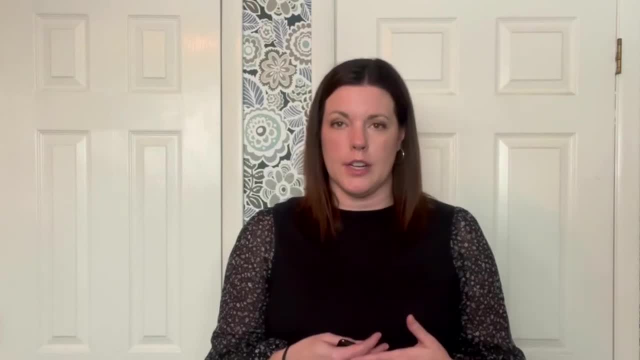 So how much was the cost of goods sold value in each of the methods for our shirt, example? Our cost of goods sold values can be seen here. As you can see, the cost of goods sold value in each of the methods is lower than the cost. 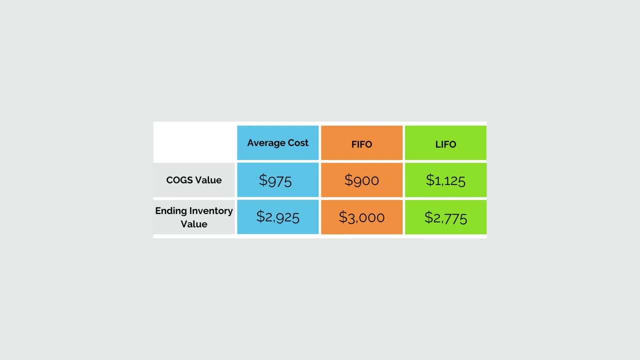 of goods sold. Similarly, the inventory method a company uses affects its cost of goods sold, which has a direct impact on profitability. If you use the FIFO method, you'll report a lower cost of goods sold, which increases your gross profit and net income.